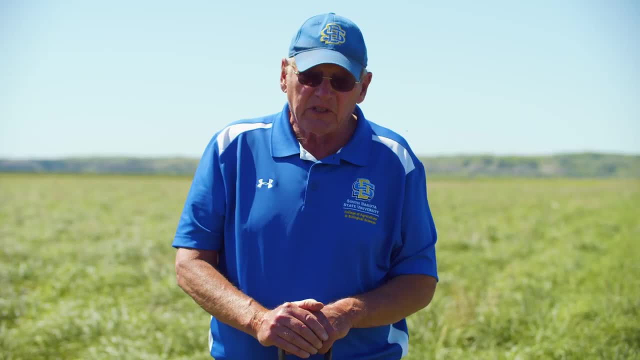 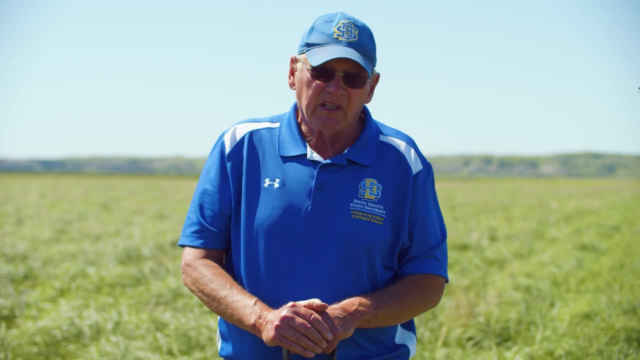 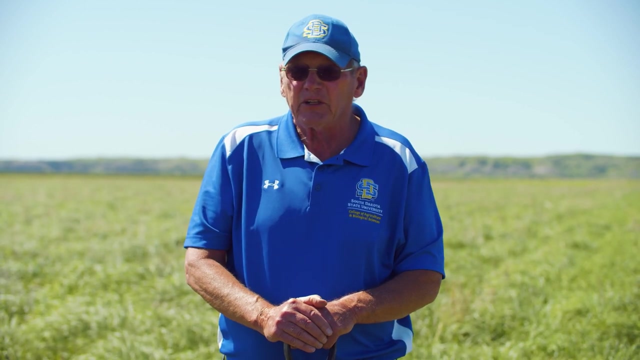 five years ago or six years ago, because it was initially an alternate year where what do we call an alternate year rotation? It went from corn to peas, to winter wheat and then soybean, So it was every other year broadleaf- Half of the crops in the rotation. 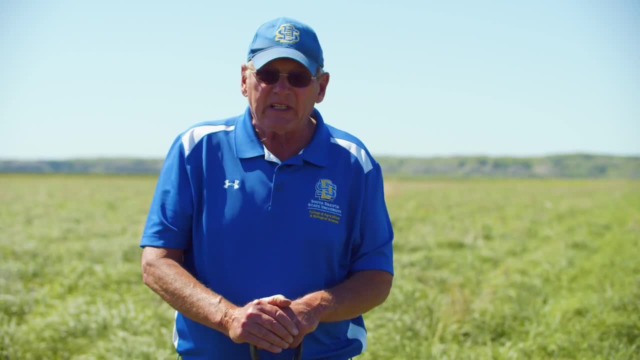 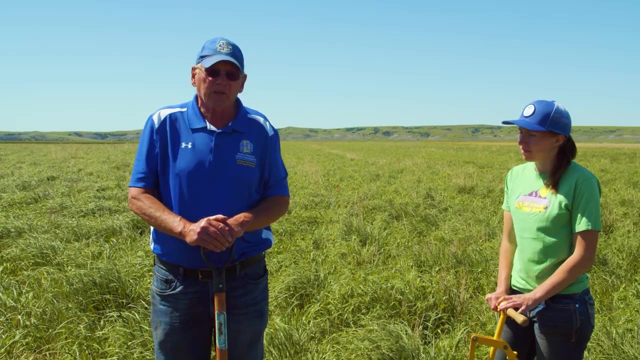 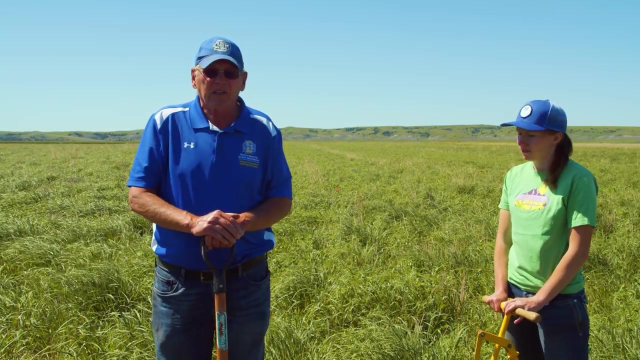 were low in carbon. There were reasons we did this, but it's very destructive to the soils and we have quite a bit of data that show wheat growing in this rotation compared to other crops. compared to wheat and the rotation across the path here will be yield half what it does. 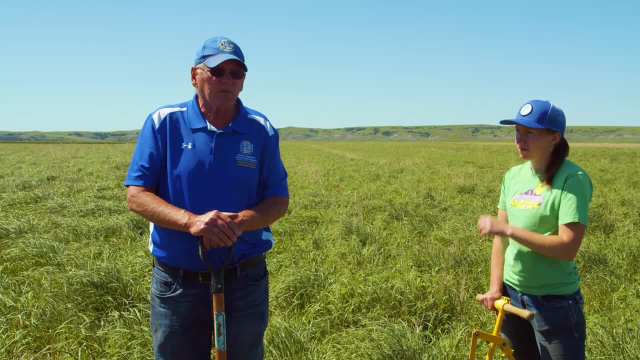 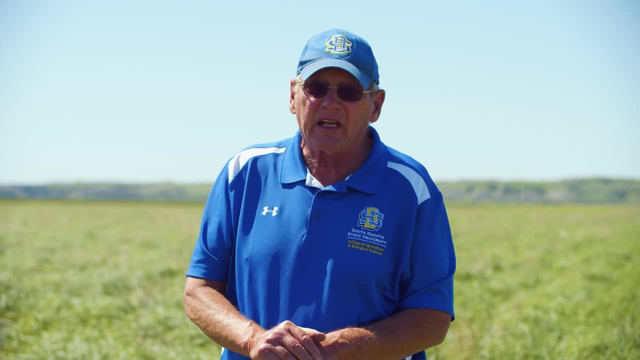 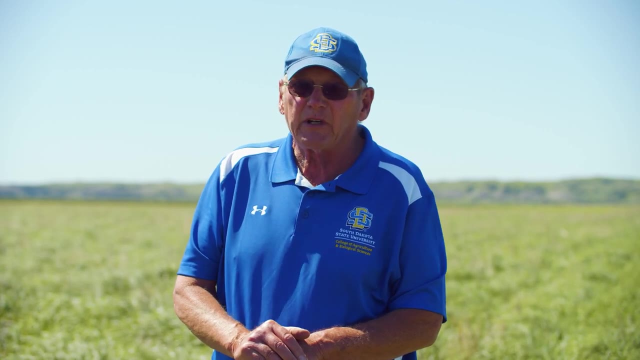 over there in challenging years, and it's simply because the soil has become less productive. Our solution to that was to add a perennial sequence, and that's what our ancestors used to do is they would farm for a while and then put it back in perennial or in the tropics, they let it. 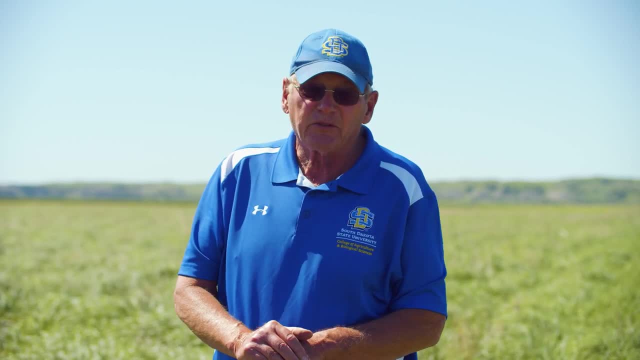 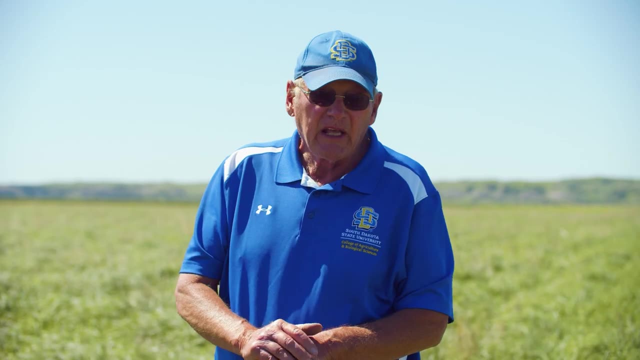 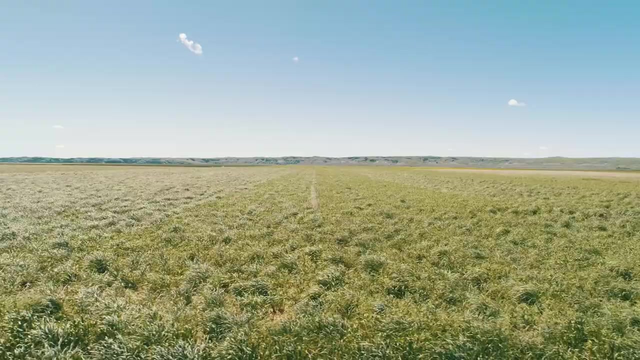 grow back to jungle. I was in Ghana a few years ago and that's the way they ran their farming systems and let it regain its fertility, so to speak. So here we're going to look at the soil. we use switchgrass as our perennial sequence. This is the last year of the switchgrass and it'll go back into an annual sequence again. 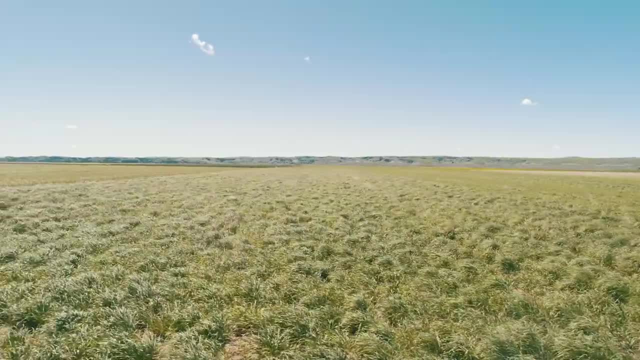 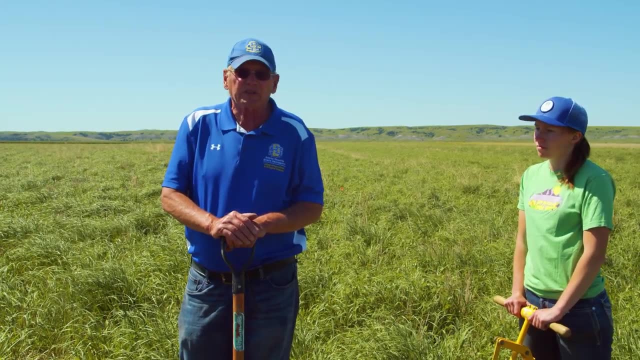 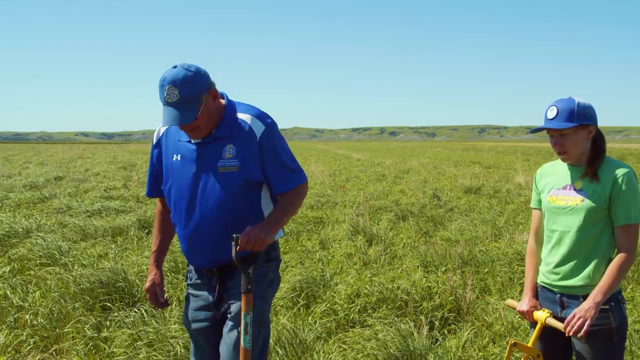 The crop we took out was the soybean, So we now have two-thirds of our crop for high residue. plus we do switchgrass as a perennial sequence and it's high in residue and has a very deep rooting system, so it brings the nutrients back up from below. 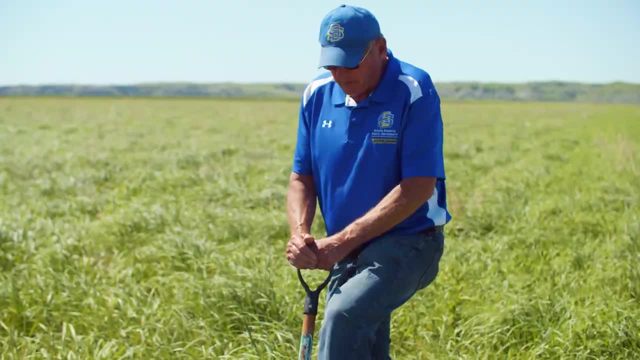 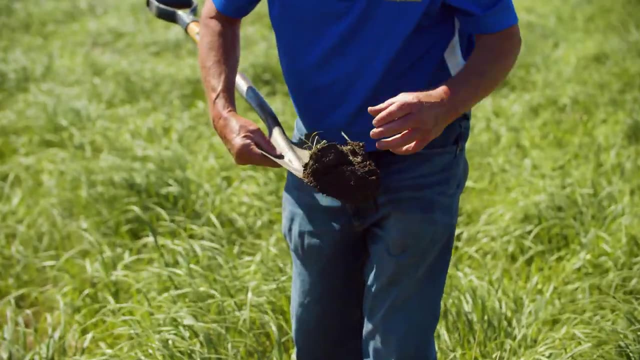 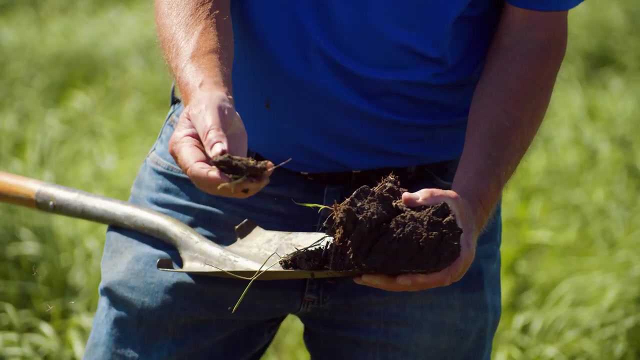 If I take these spaces between the switchgrass, it has some of the remnant that gave us problems in terms of soils. It has a real platey structure. That top will just plate off and it's smooth like that. The water doesn't really go into that well. 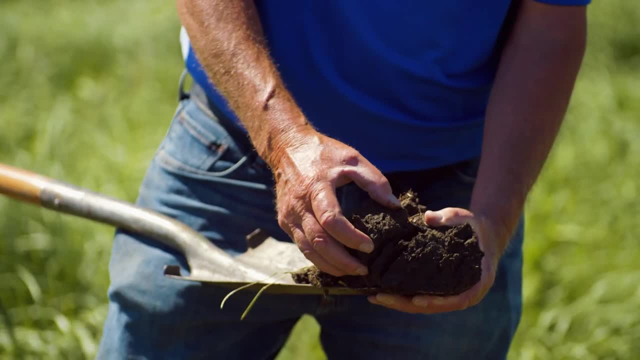 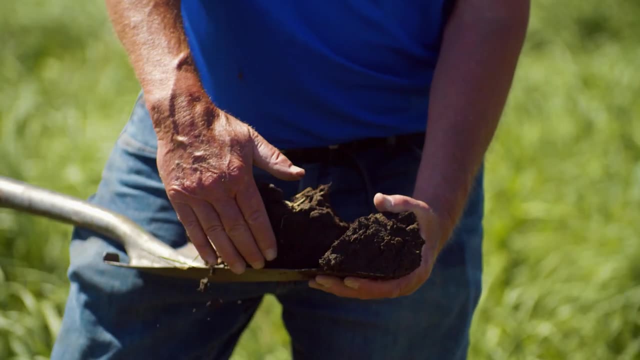 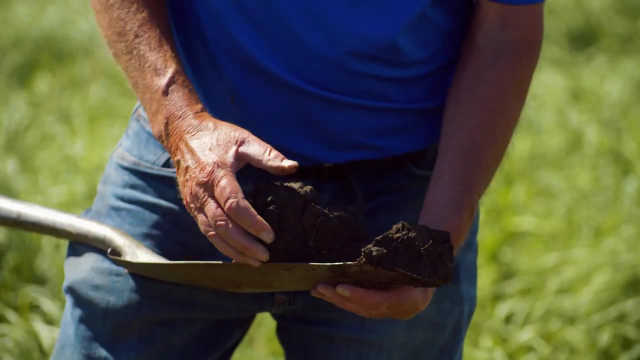 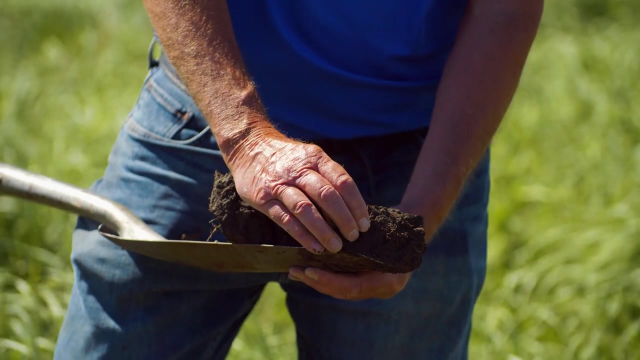 The water has to have holes to go in. It's starting to develop some macropores, but you notice right here how that whole soil just divides in a horizontal plate and they used to call that a plow pan. but it happens just because there isn't enough organic matter to hold it into a better form and there's another plate that came. 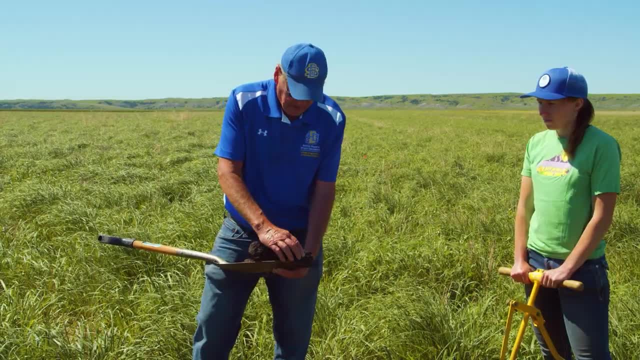 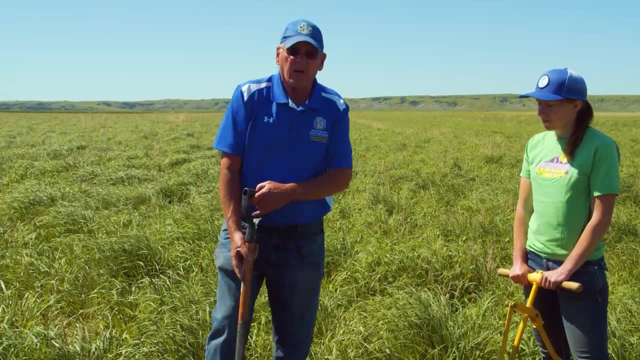 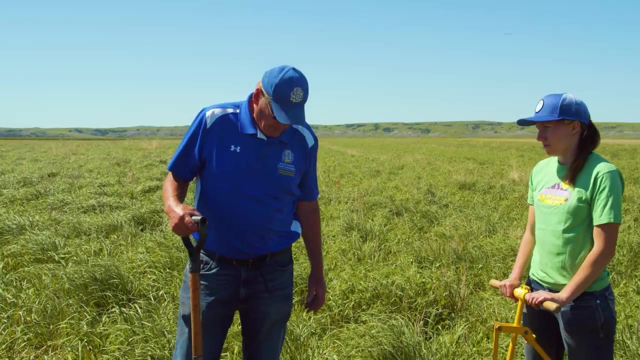 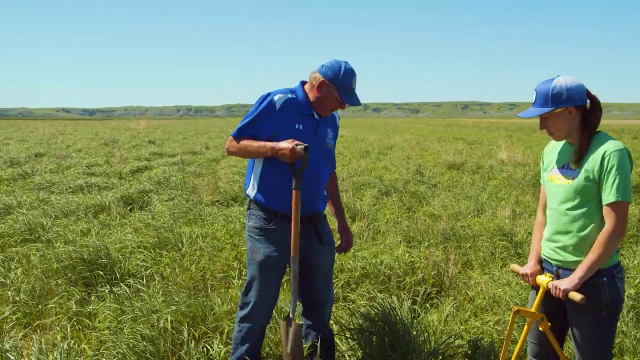 off just the same way. Now, what we started with here when we came to the prairies and Lewis and Clark actually walked across our farm just south of here along the river in 1804, or Lewis did, Clark didn't- By putting the switchgrass in, we develop a totally different type of soil structure. 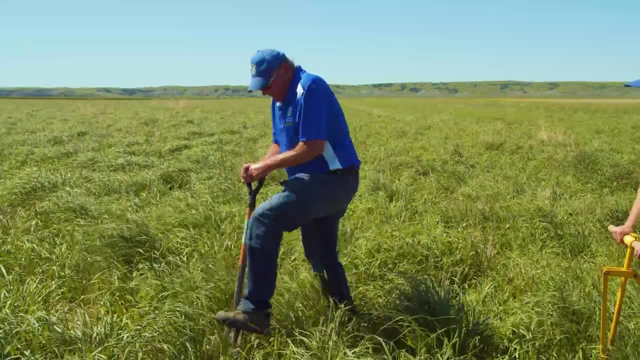 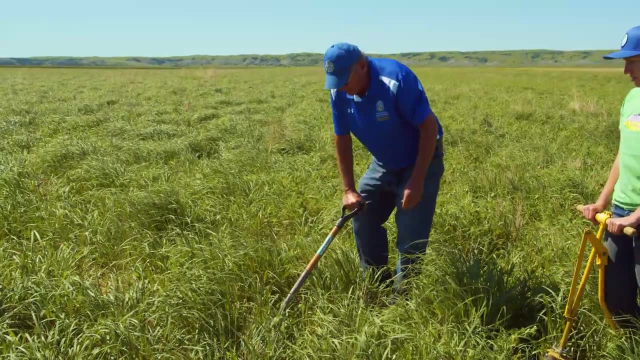 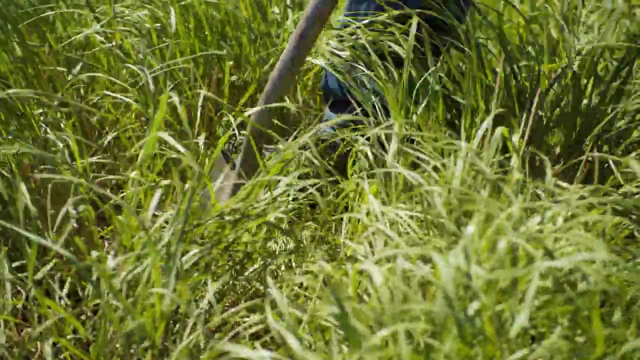 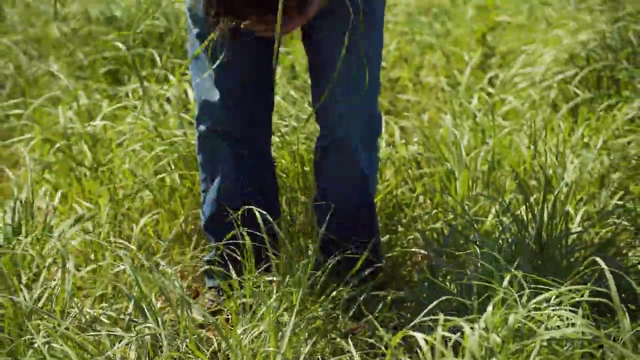 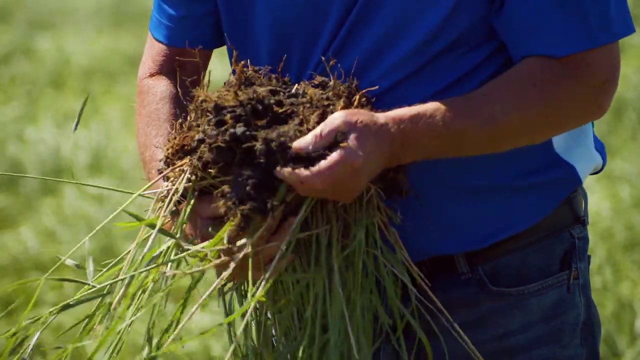 Trying to find the victim here. Now, one of the things that you may or may not be able to hear is the roots tearing. Now you see a totally different change. Now you see a totally different change. Now you see a totally different change. 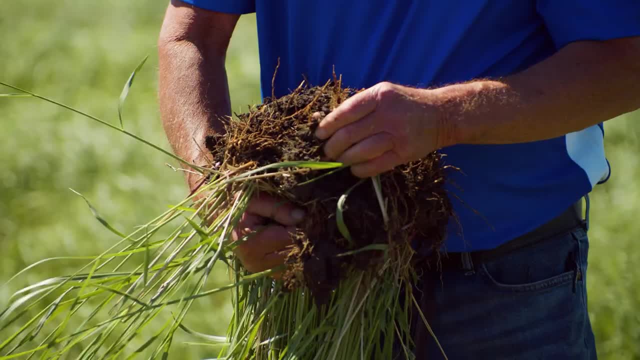 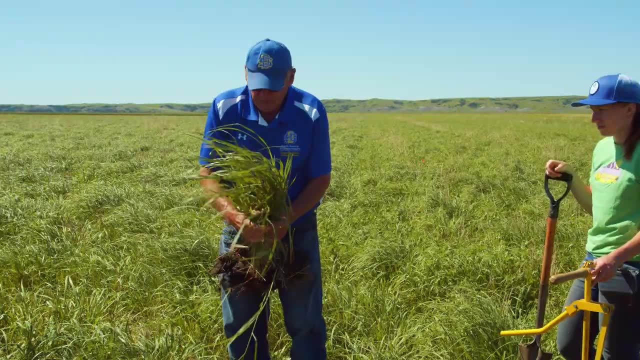 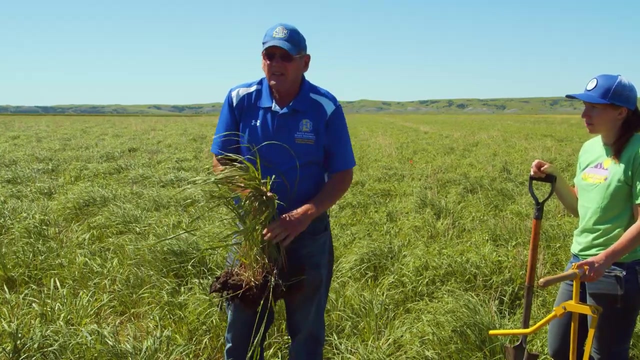 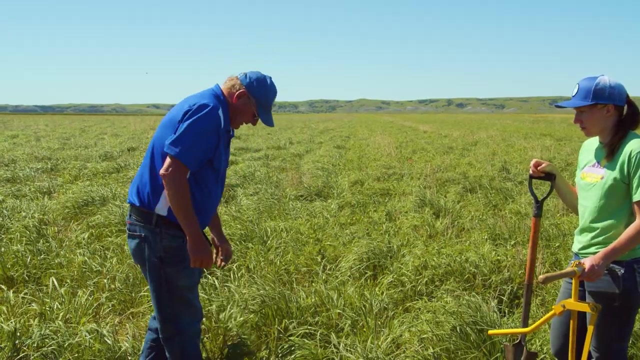 And these roots will go six to seven or eight feet deep, And so they will bring lime and gypsum and other nutrients that are trying to escape out the bottom. It will bring them back to the surface and deposit them on the surface- This part of the field we've made grass seed on for the last year. 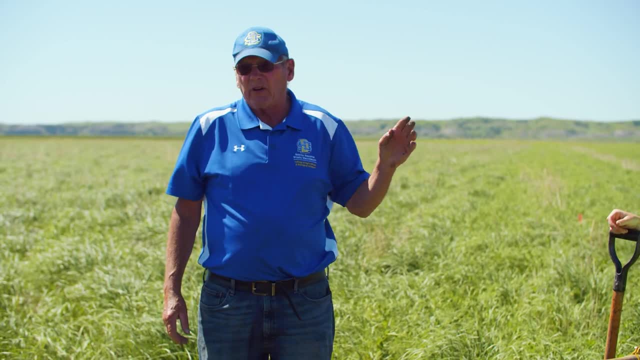 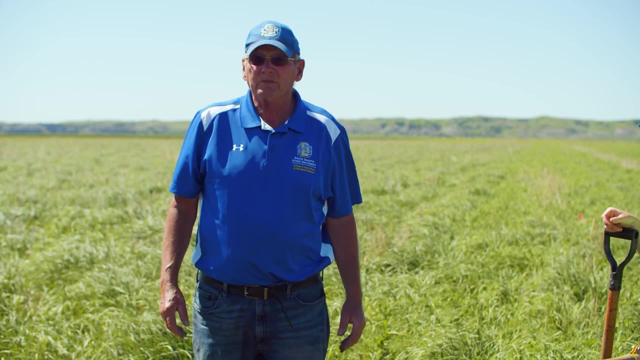 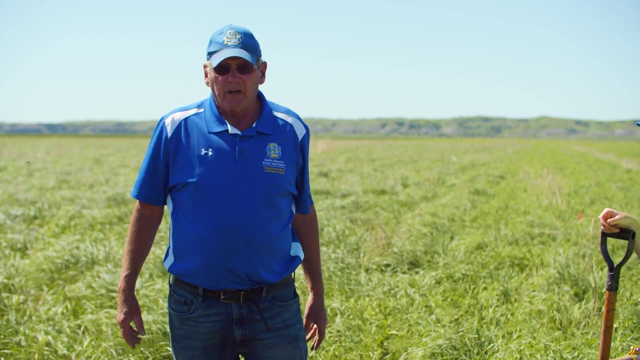 For the last number of years, the west part of the field we've grazed, So we cycle that nutrient. most of that nutrient remains here and cycles back into the system. So we've captured it, brought it up, released it and then, starting next year, we'll go to 15 years of an annual cropping.